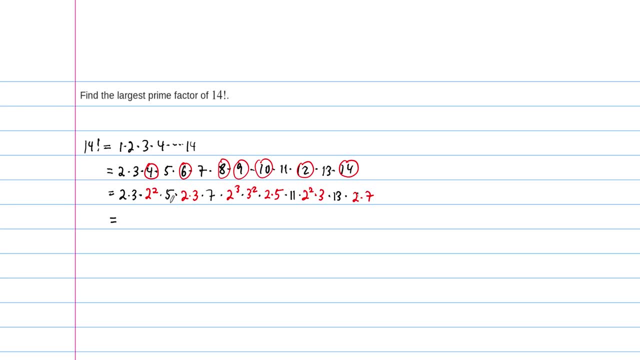 Right, So we have 1,, 2,, 3,, 4,, 5,, 6,, 7,, 8,, 9,, 10,, 11.. So this is 2 to the 11th power times. 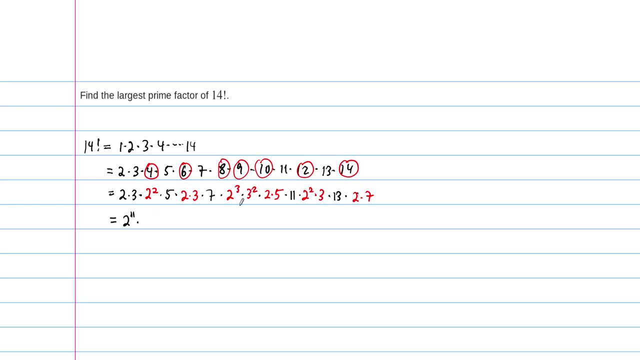 Now count the 3's. So 3's we have 1, 2, 3,, 4, 5.. So this is 3 to the 5th power. Now the 5's: There's 1,, 2, 5's. 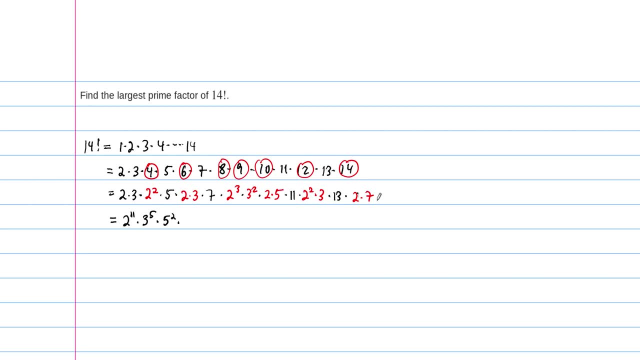 Right. So 5 squared 7, there's 2 sevens, So 7 squared, And then the rest of the prime, So then 11 times 13.. So there's the complete prime factorization of the number 14 factorial. 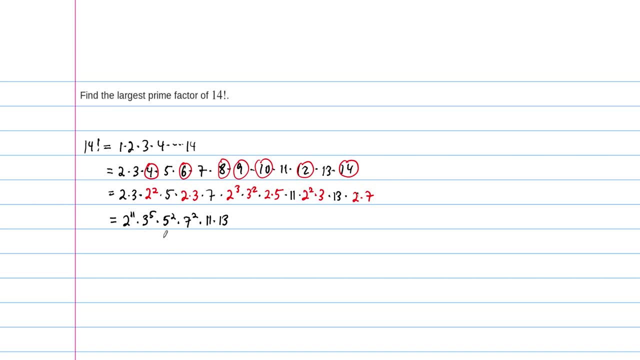 By the way, this number is huge, Right? In case you had any doubts about this, 2 to the 11th power is already 2048, right? so 2048 is the first factor here, and then multiply by all these other numbers, so this number is gigantic, right? 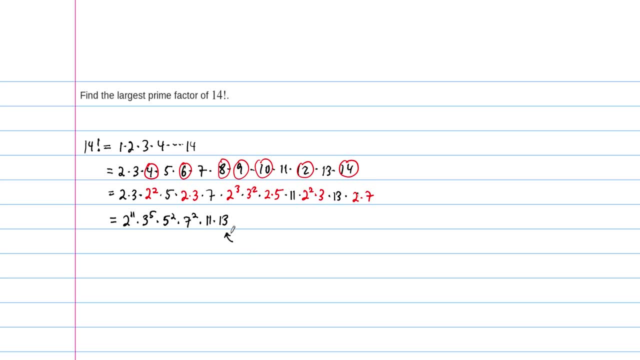 but the largest prime factor of this number is just 13. so, to answer this question, the answer is that it's 13. that's because of how the numbers built, but it's also a good idea to write out the entire prime factorization of this number. 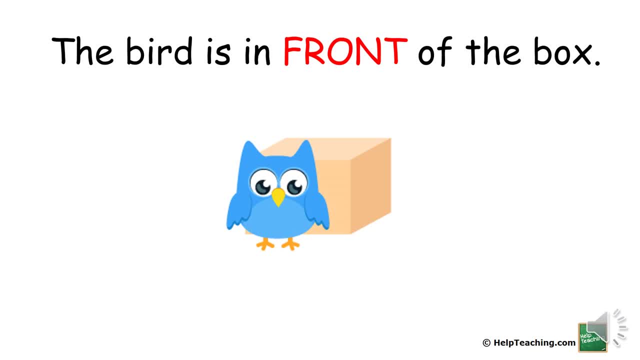 The bird is in front of the box. The bird is behind the box. The bird is above the box. The bird is under the box. The bird is in the box. The bird is on the box. The birds are next to each other. 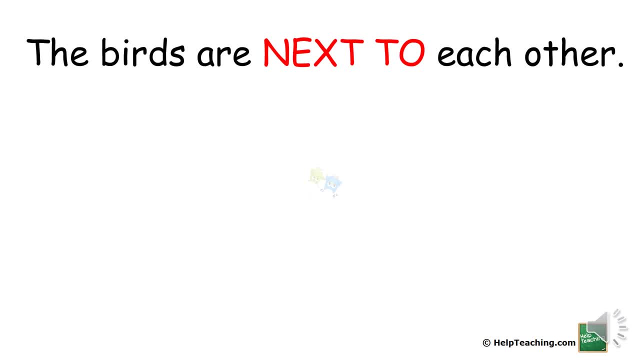 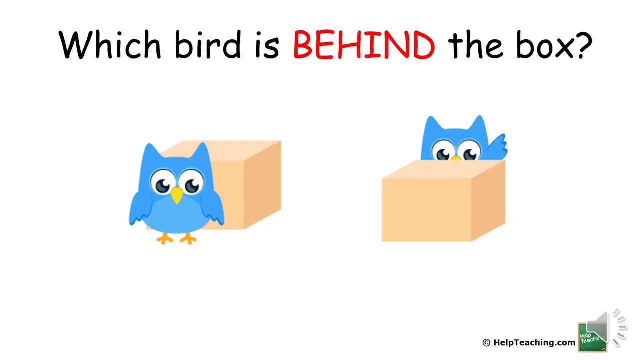 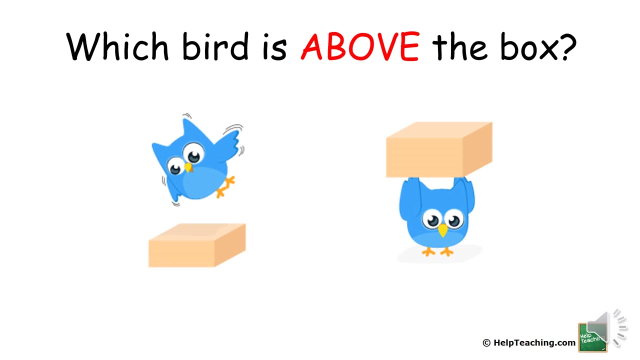 The birds are next to each other. Which bird is behind the box? Which bird is above the box? Which bird is next to each other? The bird is behind the box. The bird is next to each other. The bird is on the box.